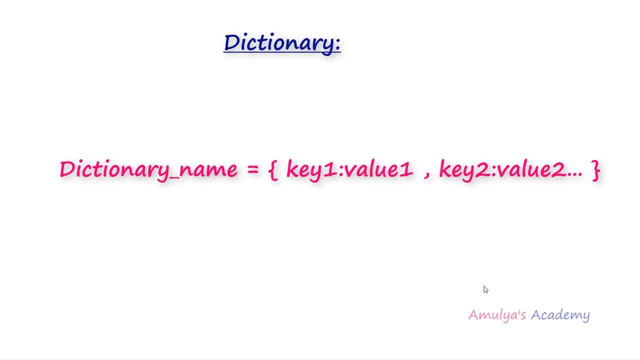 this. We need a dictionary name, followed by the curly brace and we have key and value pair. Key and value will be separated by colon and each key value pair will be separated by the comma. So here keys in the dictionaries need to be unique and we can have only immutable objects. 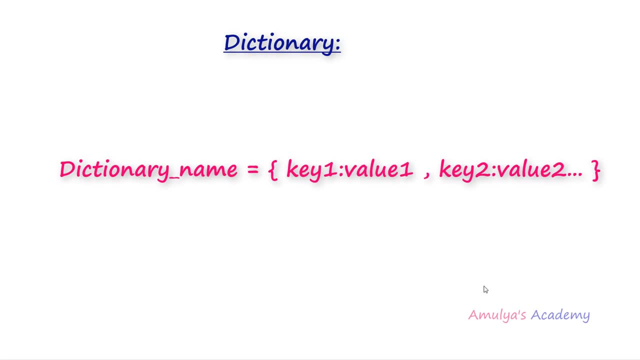 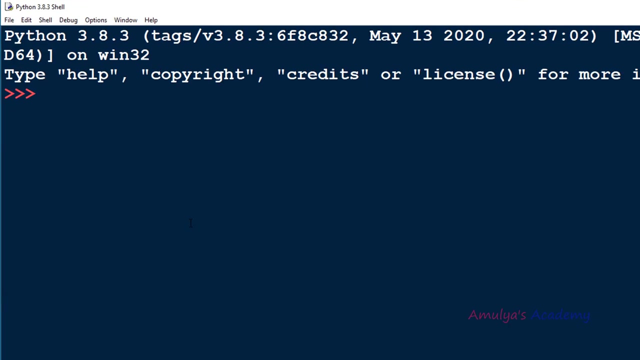 as key Values can be mutable or immutable, but keys must be immutable objects. That is nothing. but we can't have list as the key of a dictionary. Alright, so let's see how to create the dictionary and how to use the dictionary. So, to create the dictionary, we can use the. 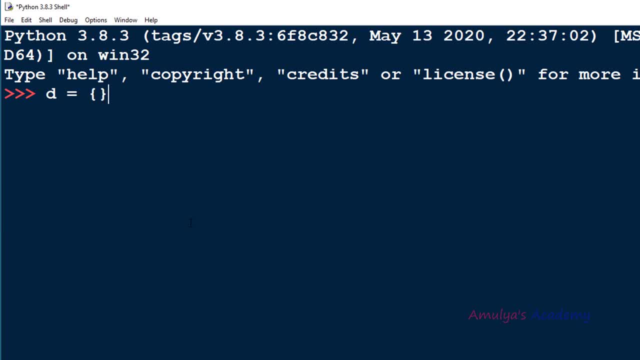 dictionary name followed by the curly braces. If i do this here, we are creating an empty dictionary. So now, if i check here, we can see D is a dictionary and it doesn't contain any elements. that means it is a empty dictionary. or if you want to create a dictionary with key and value pair, you can take like this: 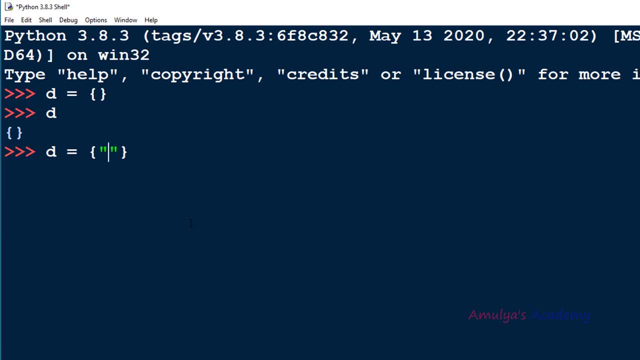 In the dictionary within the curly braces. i will take key as string here. so i will take name and here i will take value as email address, again a string value, something like this. ok, So now if i check D here, we can see It contains key, value pair and the key and values are separated by the colon and key. 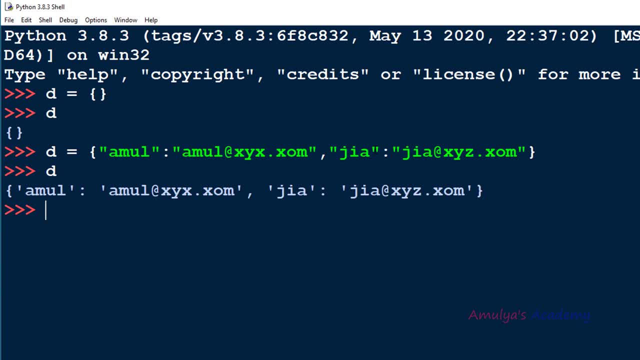 and value pairs are separated by the comma, And also you can create the dictionary using dict constructor. So now D will be an empty dictionary. Ok, in this way we can create the dictionary in python. As i said, in the dictionary keys are unique. You can't have duplicate keys. 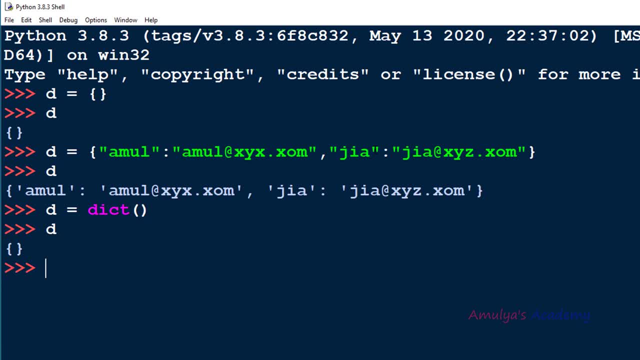 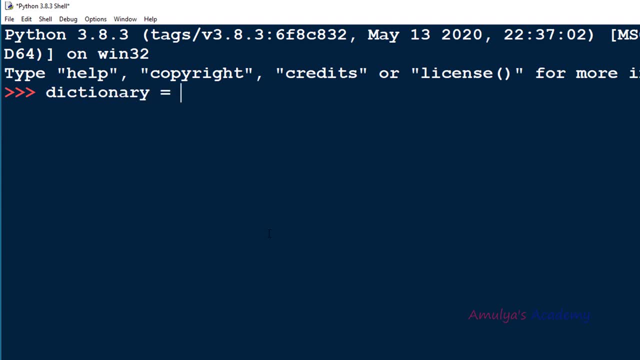 For example, if you have duplicate keys, what will happen? I will show you that. So here i will create my dictionary. as dictionary equal to, here i will take: j is equal to 1, and again i will take key as j and here i will take value as 3, right. So now, if i see the dictionary, here we can. 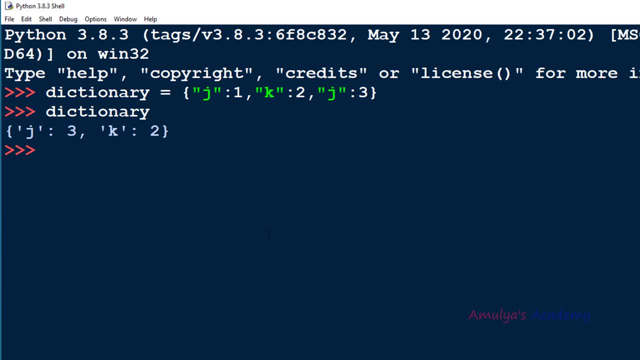 see j is 3 and k as 2.. Here we can't see the duplicate key. that will be removed from the dictionary. So here i will create my dictionary as dictionary and we can see that the key is removed and 3 is assigned as the value for the key j. 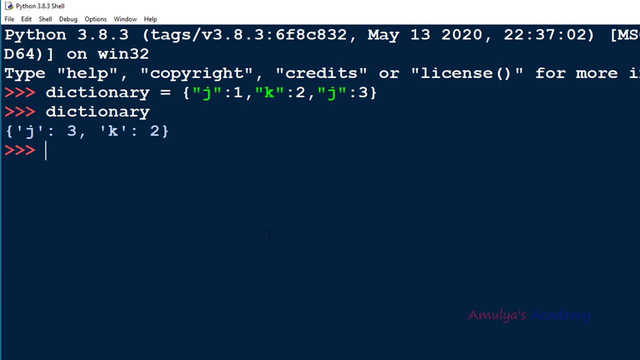 Keys in the dictionary need to be unique and also, as i said, we can't use mutable objects as key. For example, if i create a dictionary and in this, if i use a list like this as the key, we will get error. ok, so we can't use the mutable types, as key Values can be mutable. 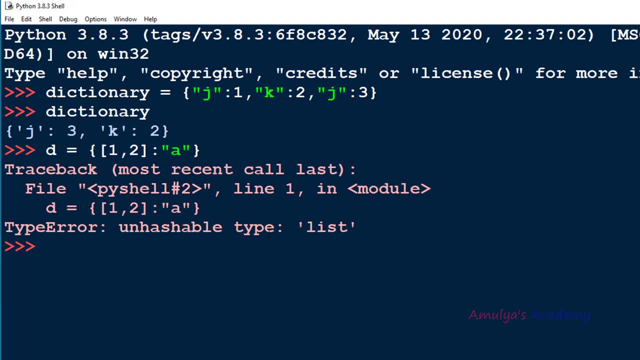 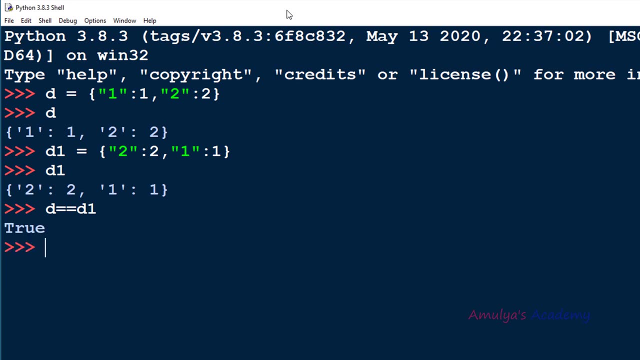 type or mutable type. that is ok, but for key you need to use the immutable objects. You can use strings tuple like that. Next, dictionaries are unordered. Now if i check whether d is equal to d1, yes, it is true. Dictionary is not ordered. If you want to organize the 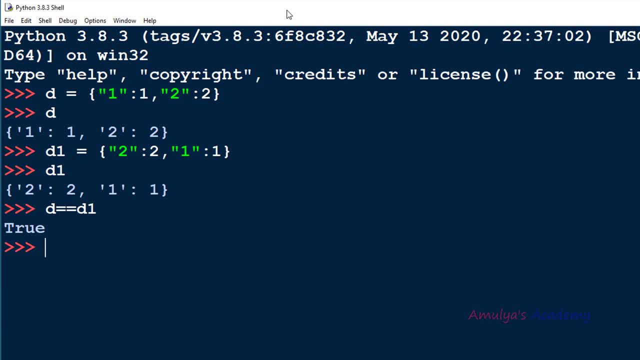 data. you can sort this manually, but dictionaries are unordered. And next, because dictionary is unordered, you can't access the element from the dictionary. so you need to use the key to access the element from the dictionary. For example, here we have a dictionary, so now if i want to access value 1, i need to use d and square brackets in that. 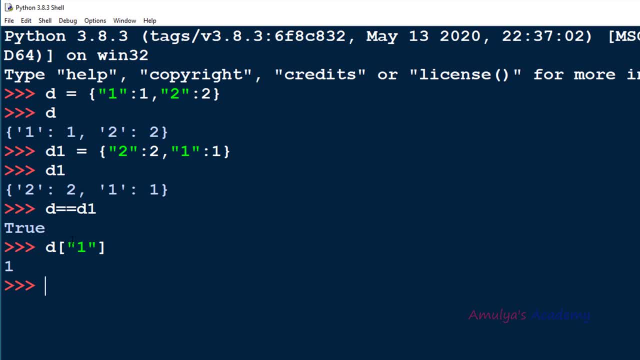 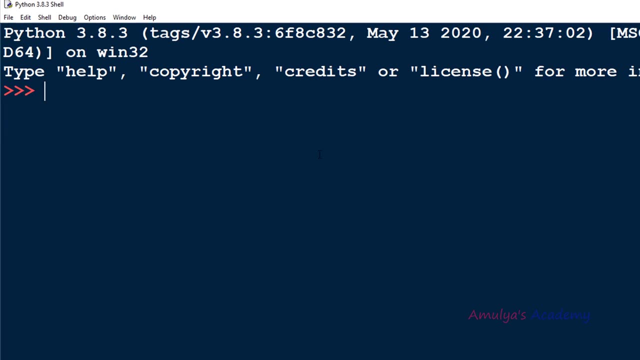 i need to mention the key. It will allow us to access the element. If you want to delete the elements also, you need to access the value using the key. like this, right And dictionaries are mutable, So you can add or delete the element from the dictionary after creating that, For example. 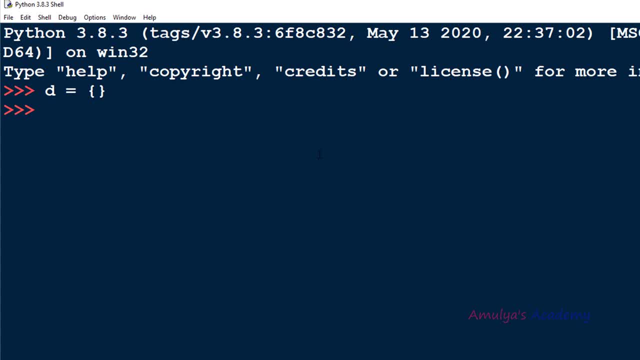 if i have a empty dictionary. now i can add the element to the dictionary using key. I need to write like this: d, and here i need to mention the key. for example, if i take key as 1 and equal to, i need to write the value. Now, if i check here, we can see And you can. 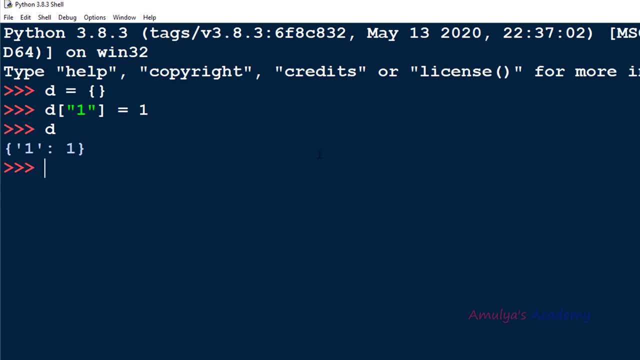 delete the element from the dictionary also. so dictionaries are mutable, Dictionaries can be nested, so you can use dictionary as the value of another dictionary. You can't use dictionary as the key of another dictionary because, as we know, key can't be mutable object right, But you can use a dictionary as the value for another dictionary, For example: 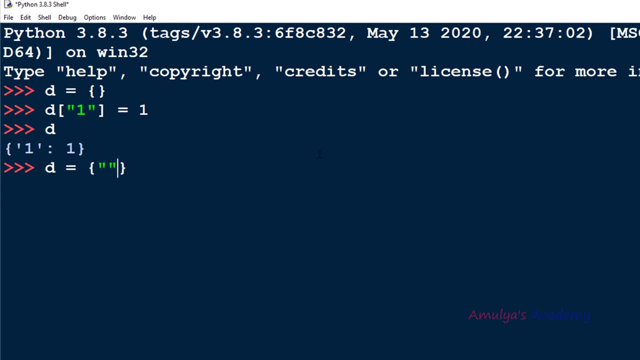 here i can take 1 equal to. here i can take value as another dictionary, Something like this: ok, Ok, this is allowed. Ok, so this is about the dictionary. If you want detailed explanation of the dictionary, then you can go and watch my previous videos. The video link is in the 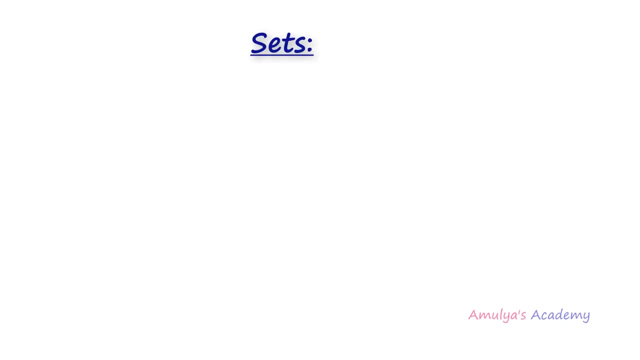 description box. Alright, so next we will talk about the set data structure. So set is the collection of unique elements. So in set no item can be repeated. Set is the collection of unique elements. You can't have duplicate values in the set. 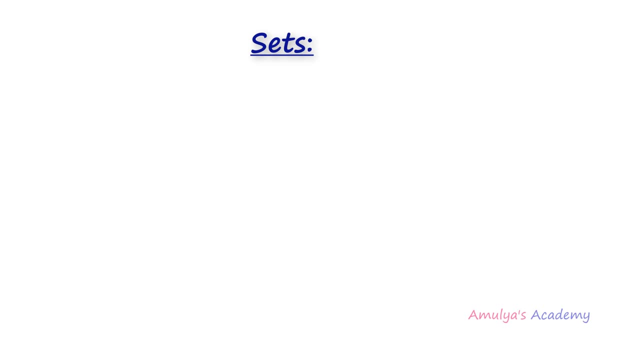 Set can be defined using the curly braces. Yes, both the set and dictionaries can be defined using the curly braces, But the syntax of both data structure is entirely different. right In the dictionary we have key value pair, but in the set we don't have that. But 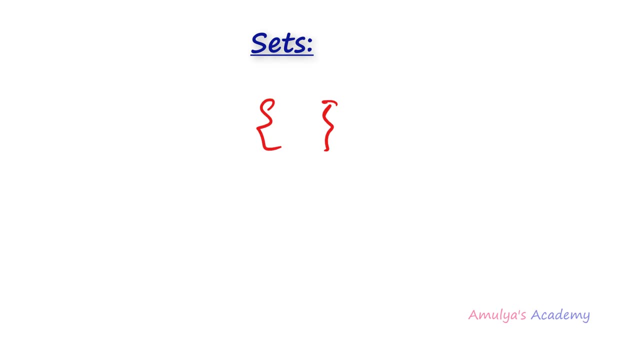 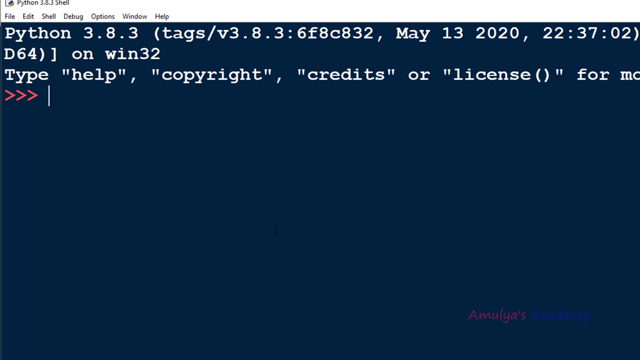 this curly braces without any element denotes the empty dictionary. To create the empty set you need to use set constructor. So let's see how to create this set. So, as i said, if you want to create an empty set, you need to use the set constructor. So here i will take 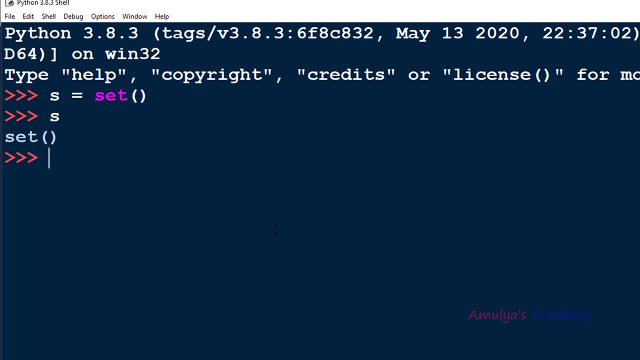 yes, equal to set, and here we can see. Or you can create the set from the string. For example, here i can take set, or here i can take string. Ok, or i can use right, Like this, Or you can create using curly braces also, For example like this: It is a set. 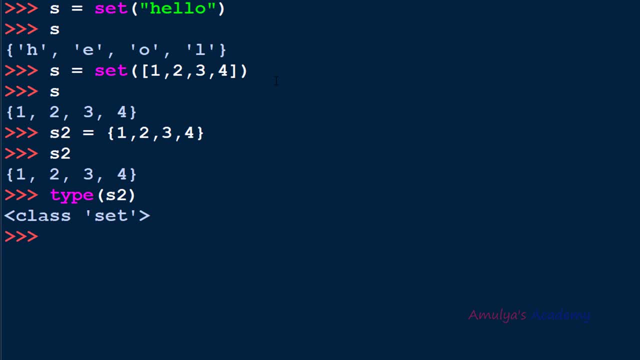 If you are taking the curly braces and inside that if you are taking key value pair, then that means that is the dictionary In the curly braces. if you are taking the elements, then that is the set. Alright, so next, As i said, set is the collection of unique element. 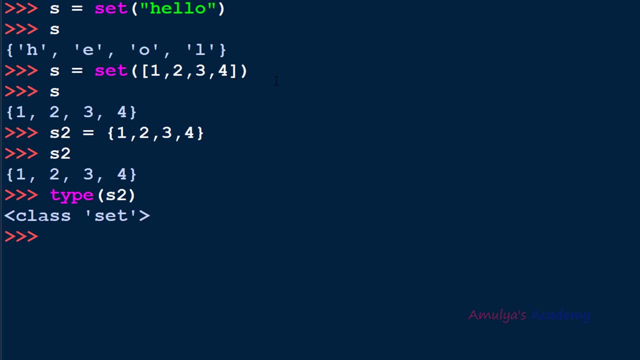 It doesn't contain any duplicate values. So what happens if i use the duplicate values? For example, i will take like this, and in the curly braces i will take values like this: Right and i will enter. Next i will see: yes, Here we can see 1, 2, 3.. It won't accept the 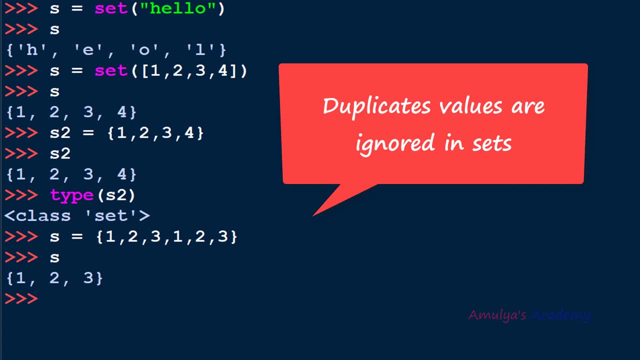 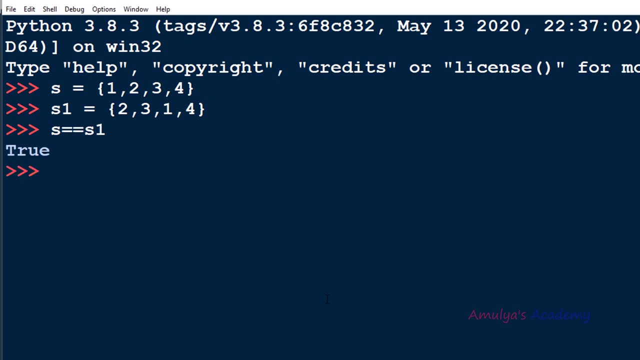 duplicate values. Set is also unordered, Like dictionary set is also unordered. If i check, S equal to S1, it is true. ok, Set is mutable. So after creating the set, you can manipulate that. You can add elements or you can delete elements from the set. To add the element, you can use add method. So 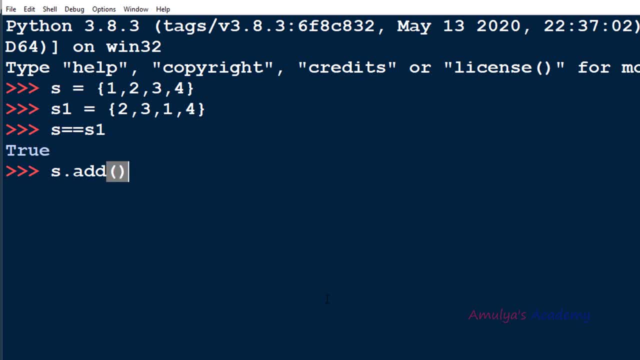 for example, you can take S, dot add and here you can add the element. Still i get 1, 2, 3, 4 because tree is already present, so it won't take the duplicate values. But if i add set, here we can see. So set is mutable. Set can contain only immutable obj as elements. 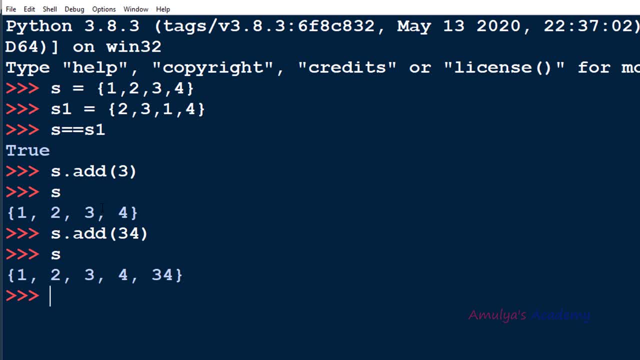 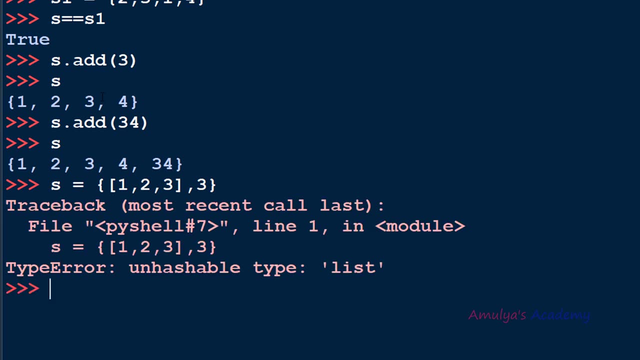 Mutable types cannot be element of this set. So that is nothing. but you can't have list as the element of set. Set can have only immutable object as elements. For example, if i take like this, we will get error. Set can contains only immutable type elements. 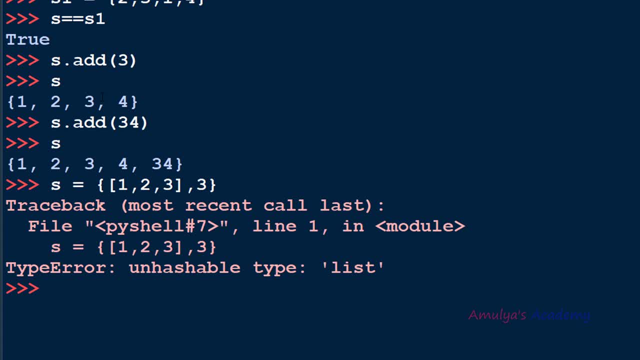 elements. so that's why set cannot be nested. we can't have set inside a set, because set is mutable right, it is a mutable object. so that's why we can't have set as the element of another set. so set can't be nested. for example, if i have inside that i'll have one. 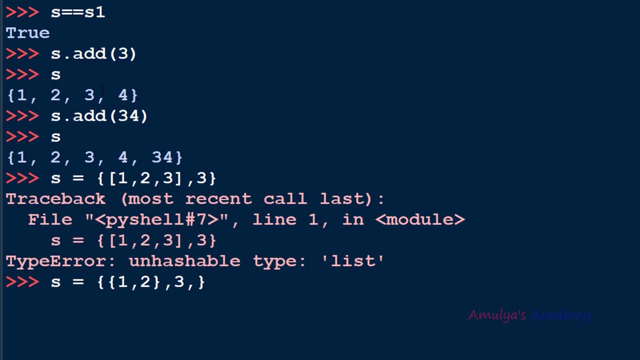 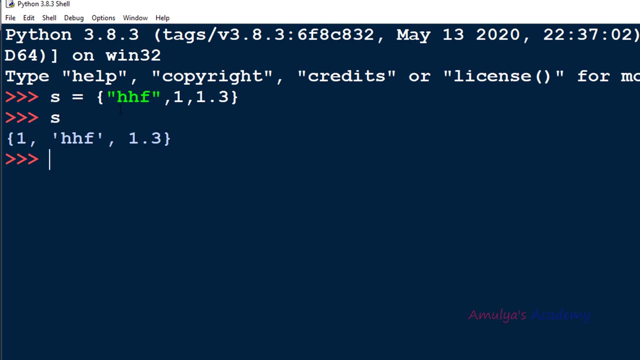 two, we'll get error. set can have different types of element, but the type of element should be immutable objects and you can perform the standard operation of this set which you use in the mathematics here also, like union, intersection, difference etc. if you want to create a list. 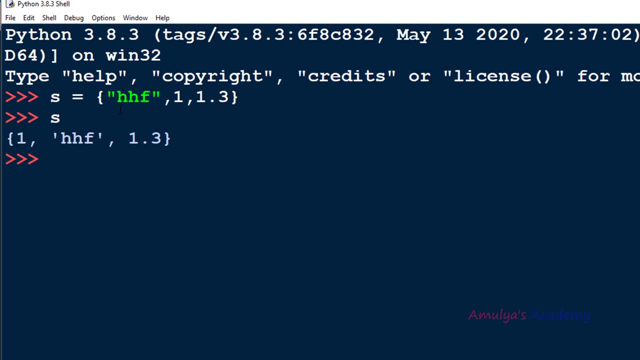 of items where each element need to be unique, then you can use the set data structure and because set is unordered, we can't access the element from set using the index. in the dictionary we have key value pair and using key we can access the value, but in 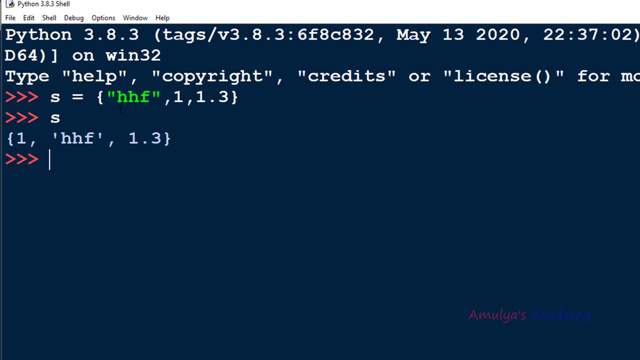 the set. we don't have key and value pair also, so to access the element from the key you can use the loops, or you can check whether that element is present in the set or not using the in membership operator, for example. here you can type one in: yes, It will give.